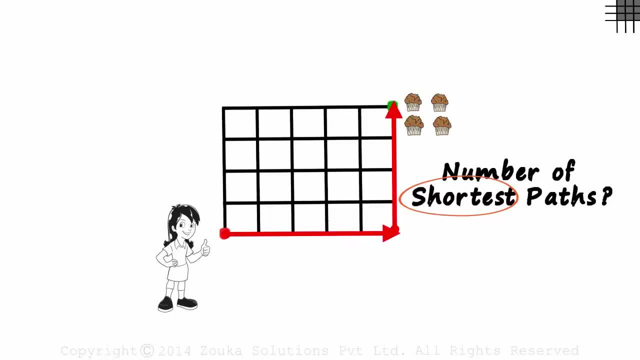 Many students assume that going to the right and then straight up is one of the shortest paths, And the other is going straight up to the right to reach the cake shop. So let's find the number of shortest paths. How do we find the number of shortest paths? 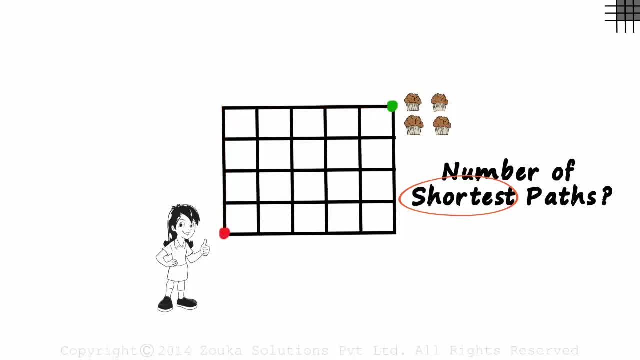 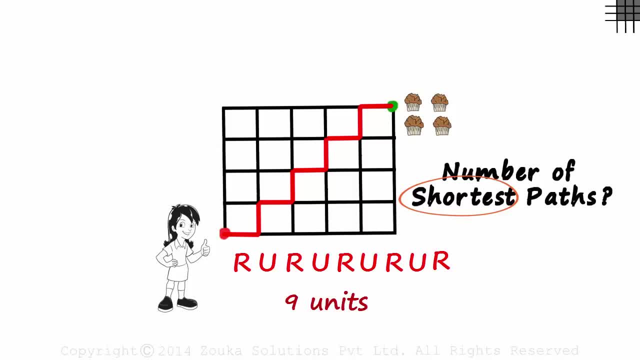 We covered 9 units lengths when we took this path. Let's take another random path: Up up, right, right Up, right up, right, right. Again, 9 units. Now let's look at the earlier paths that had crossed our minds as the shortest paths. 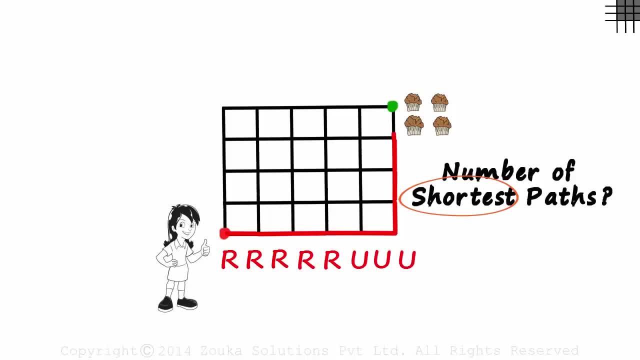 Right, right, right, Right, right, up, up, up and up Again: 9 units. We had also thought of up, up, up, up, right, right, right, right and right. The shortest path will cover 9 units. That's our conclusion. We will come back to this point in the next lesson. 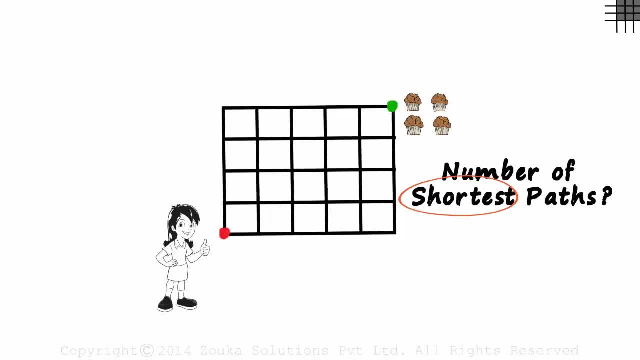 But let's answer a question that some of you all would be wondering about: What is not a shortest path? The answer is simple: At any point, if you travel left or down, it will not be a shortest path. Say you go right up, left, up, up up, right, right, right, right and right. 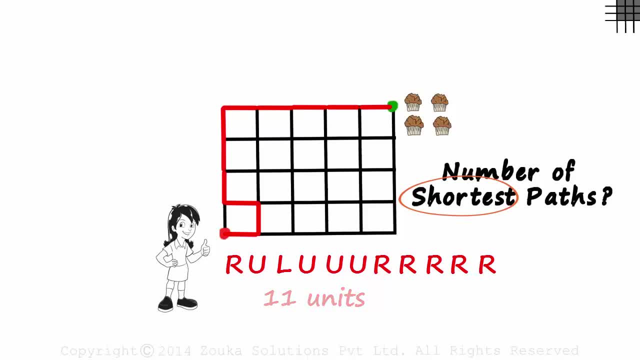 This will be 11 units and it's clearly longer than 9.. It's because we took a left here. The same logic applies if we go down, Up, up, right down, right, right, right, right, up, up and up: 11 units more than 9.. 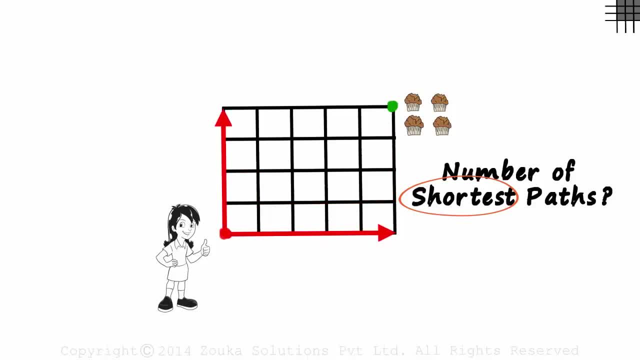 So for the shortest paths, we can either travel right or up, not left or down. Now, going back to our previous point, The shortest path will cover 9 units. What is this 9?? It is the sum of the number of columns and the number of rows. 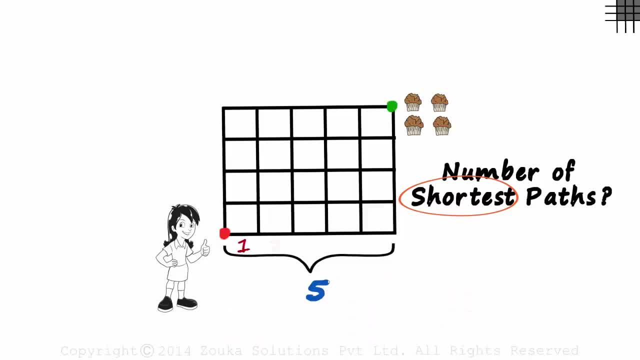 Yes, Yes, It has 5 columns: 1,, 2,, 3,, 4 and 5.. And it has 4 rows: 1,, 2,, 3 and 4.. 5 plus 4 is 9.. 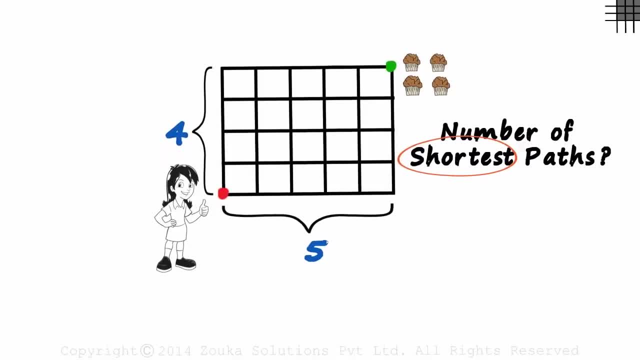 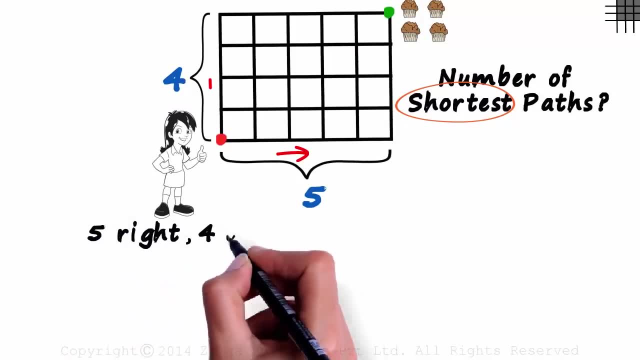 So now you know what a shortest path is. Now let's move on to solving the problem. In every case, we saw Zara had to move 5 units to the right and 4 units up. The sum of these two is 9 units. 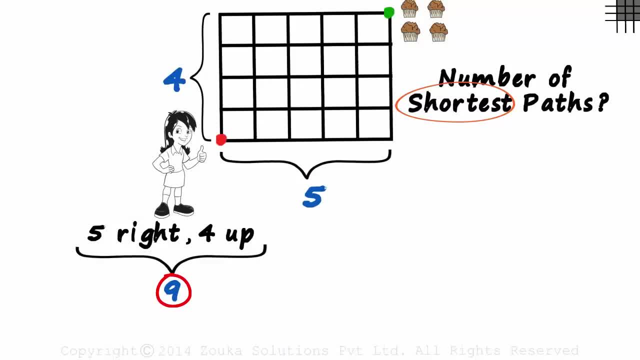 So, looking at this, can we say that out of the 9 units Zara travels to reach the destination, 5 have to be rightwards. Yes, we can say that Out of the 9 units, for any shortest path, we have to select 5 which go to the right. 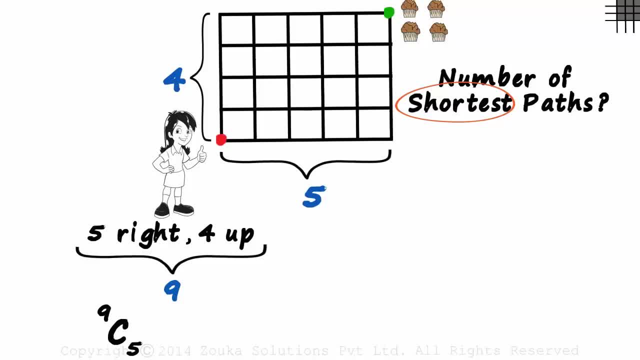 So 9C5 will give us the number of shortest paths Zara can take to reach the destination. Wait, Can we also say that out of the 9 units Zara takes for the shortest path, 4 have to be upwards? Yes, 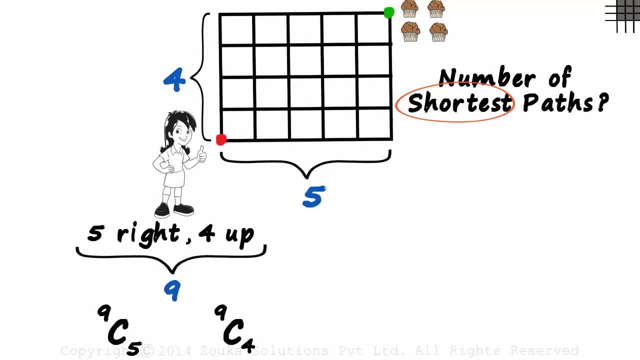 9C4 will also give us the same answer, But how? How These two will be equal. In case you are unable to recollect, the formula for NCR is N factorial divided by R factorial times N minus R factorial. This will equal 9 factorial divided by 5 factorial times 9 minus 5 factorial. 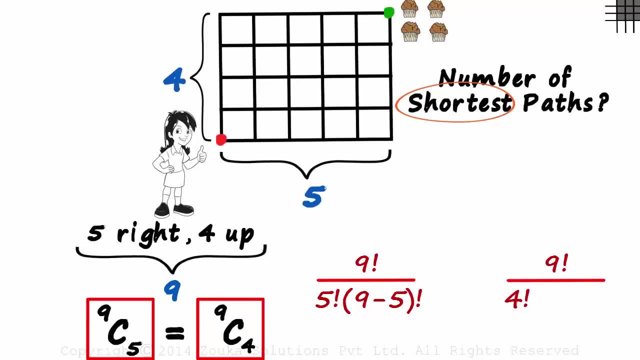 And this will be 9 factorial divided by 4 factorial times 9 minus 4 factorial- Same answer. Then we will have 26 different shortest paths Zara can take to reach the destination. Okay, we have the answer now, But is there another interesting way to arrive at this answer? 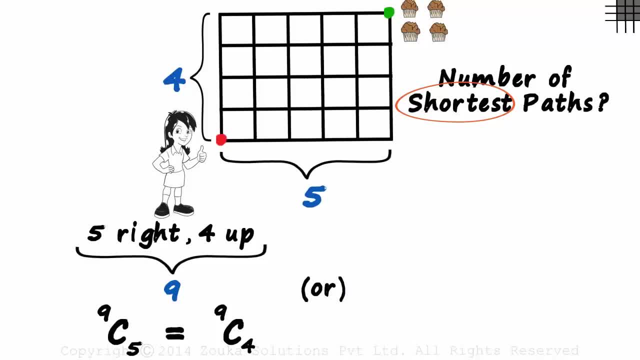 Can we use another approach we have used before? Think: Could you think of anything? Okay, So we know that Zara will be moving 5 units to the right and 4 units upwards. We know that for sure. Zara will be moving 3 units to the right and 4 units upwards. 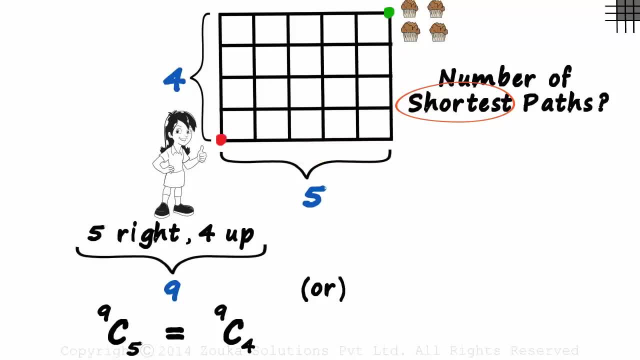 Could you imagine that? Yes, sure, No matter which shortest path she takes, it will be total of nine units, out of which five will be the del right and four will be upwards. So we write R five times and U four times. This is what we need to arrange, All possible arrangements of these nine letters.